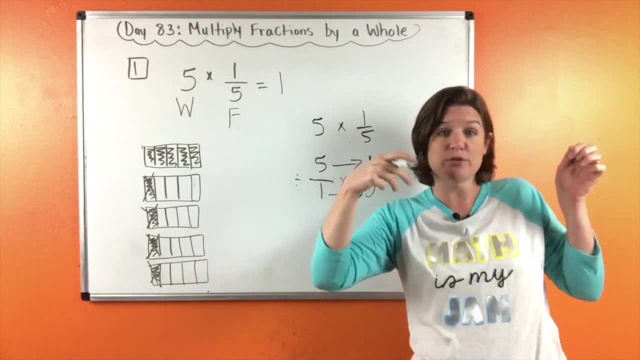 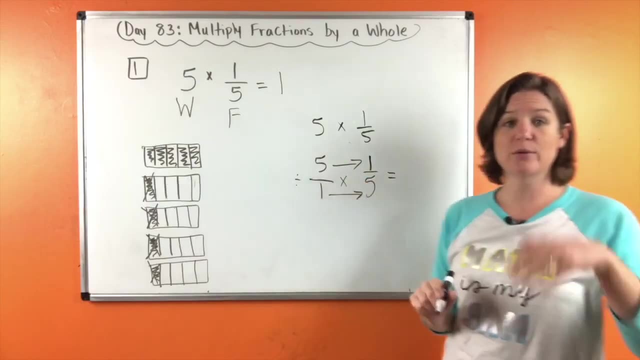 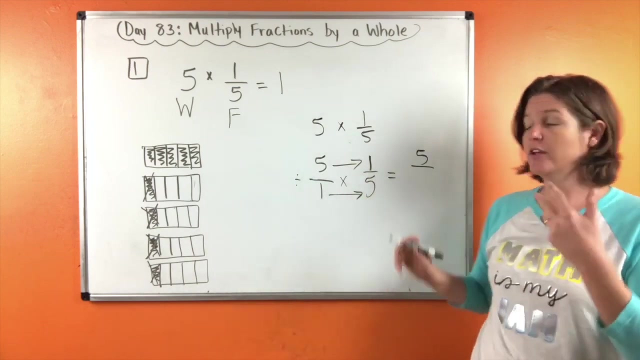 match. but when you multiply you just multiply across. It's like taking an arrow and going achoo in the numerator and achoo in the denominator. So five times one equals five and we're going to multiply across. in the denominator: One times five equals five, and five-fifths is the same thing as what. 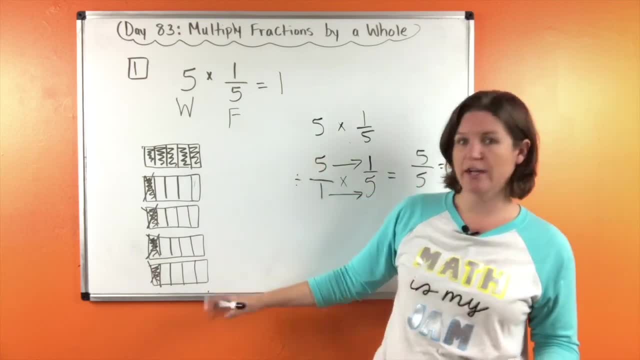 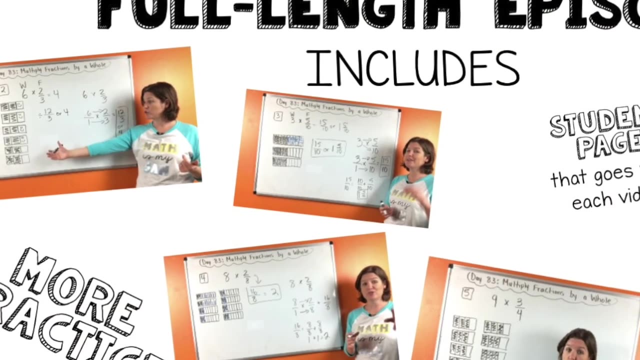 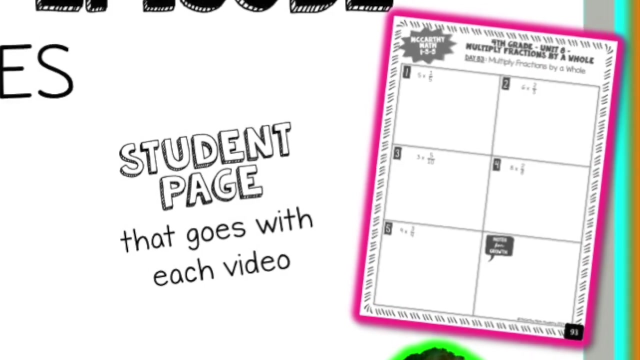 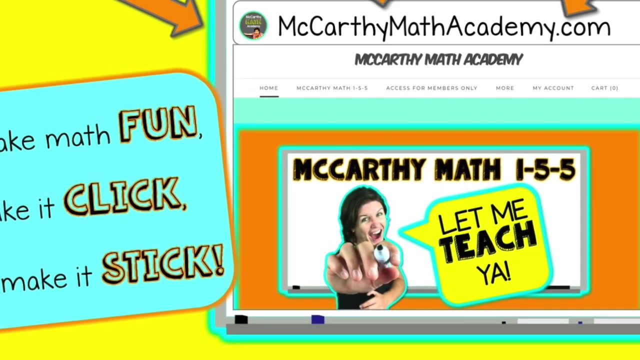 One whole, Okay. so we proved that with a drawing and we've proved it using mathematics. So our answer is one whole, All right, so we got it. Okay, we've done one And one over the other, Right? so this is just one. Right, And I think I was slightly wrong here, But I should have thought that The zero was right here, so you're right. No noise, Okay, can't hear. No stir. No liver, No here, Good, Okay. 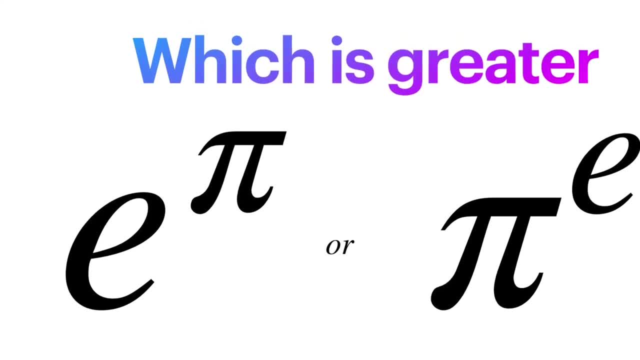 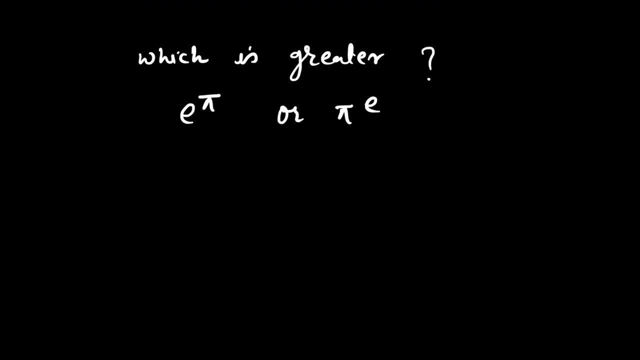 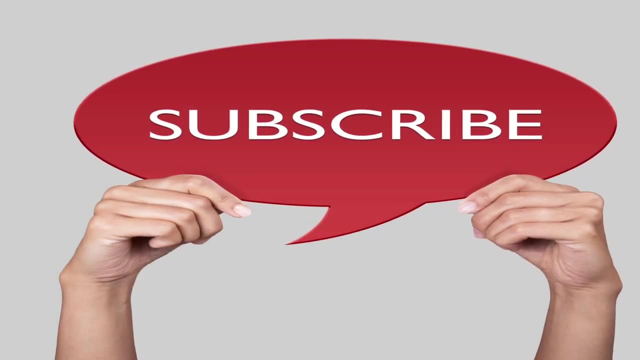 You all are most welcome in our YouTube channel, Sawal Bawal. Our question is: which is greater: e to the power pi or pi to the power e? Before I start to solve this question, please subscribe our channel and press the bell icon. You can also follow us on Telegram, WhatsApp and on. 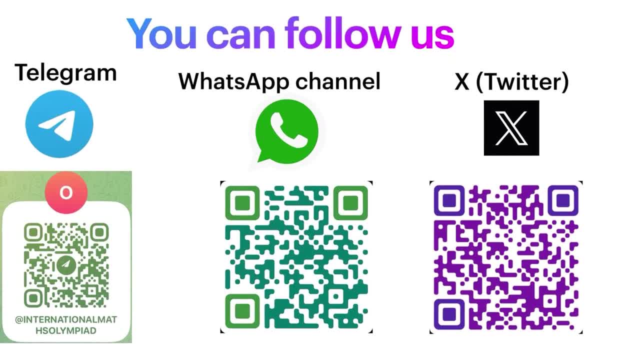 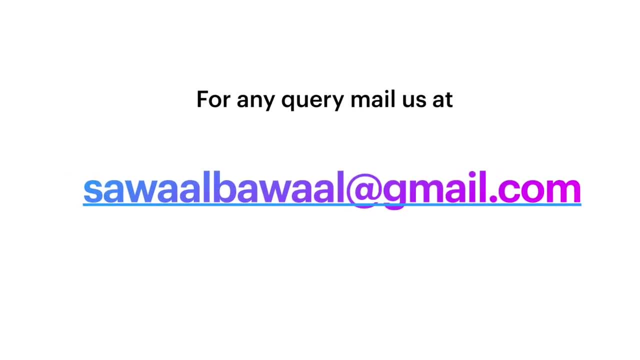 Twitter, which is now known as X. If you have any query regarding any question or you have any other question, then you can mail us at sawalbawal at the rate of gmailcom. Now let us start to solve this question. 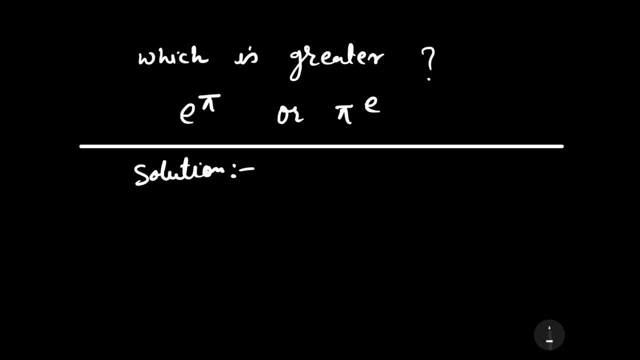 I found this question during the internet surfing. This is very interesting question. If you will try to solve it manually, then you will not be able to solve it, since the value of e to the power pi is greater than e to the power pi. So if you will try to, solve it manually, then you will not be able to solve it, since the value of e to the power pi is greater than e to the power pi. So if you will try to solve it manually, then you will not be able to solve it, since the value of e to the power pi is greater than. e to the power pi. So if you will try to solve it manually, then you will not be able to solve it, since the value of e to the power pi is greater than e to the power pi. So if you will try to solve it manually then you will not be able to solve it, since the value